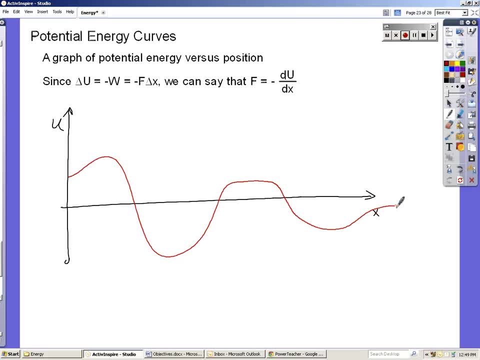 that, And it basically tells you the potential energy associated with a particular force when a particle is at different locations, And there's a lot of things we can learn about this. These graphs are one of the main tools that physicists use when we're looking at. 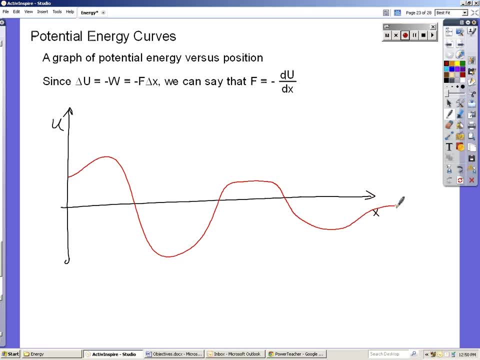 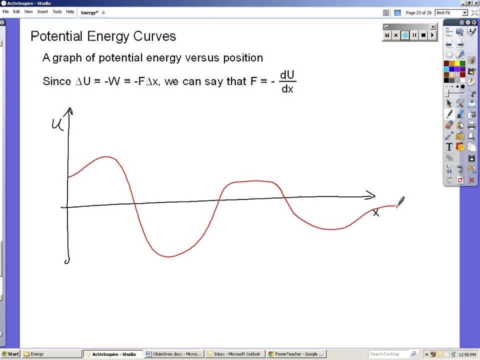 And the work is equal to the force times the displacement. So what we've got here is delta u equals negative f delta x, which, if you divide both sides by delta x and turn it into a derivative, means that the force is the negative of the derivative of this graph. 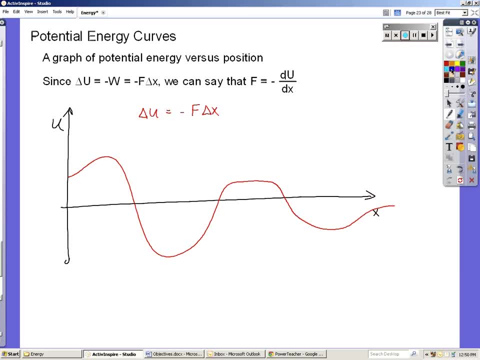 And derivative just means slope. So if you look at this point right here, the slope is negative and that means the force is positive, which means at that point the force on the particle is pushing it to larger x, Or another way of thinking about it. 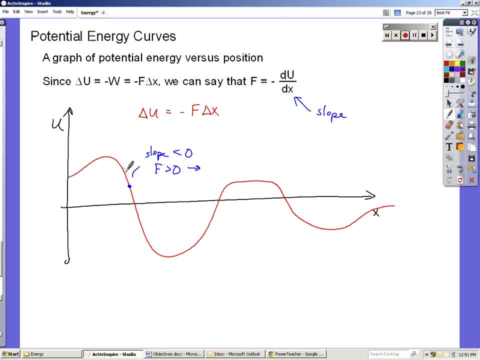 the particle wants to go downhill, So here the force is toward, is downhill, Here the force is downhill, but that means the opposite direction. Right about here the force is equal to zero, because the slope is negative, So the slope is zero. 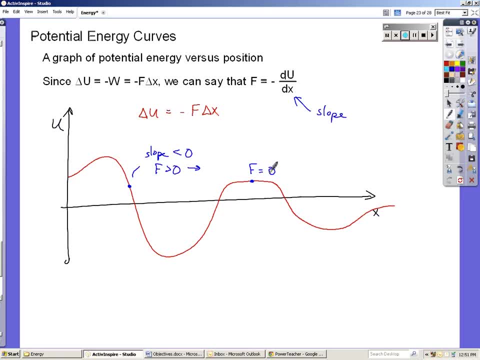 And there's a lot of things you can figure out from this. One of them is the concept of a turning point. Let's say that we have a particle, and when it is at this location here, its kinetic energy is equal to two joules. 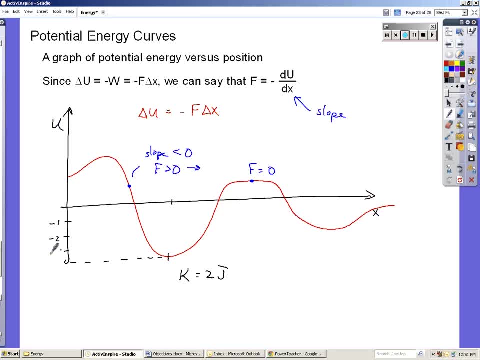 And I'll put a scale here, I'll put a number here, Let's see if I'm right. OK, The kinetic energy is equal to two joules. So, right there, the kinetic energy is two joules. The potential energy at this point is negative four joules. 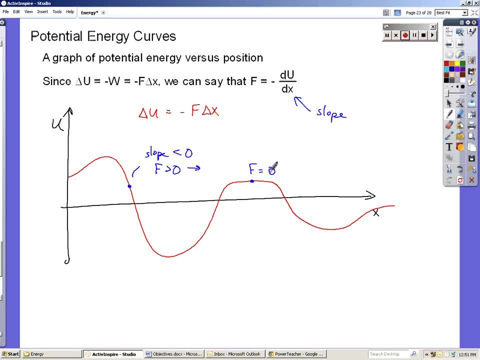 Let's say that we have a particle and when it is at this location here, its kinetic energy is equal to two joules, And I'll put a scale here. So, right there, the kinetic energy is two joules. The potential energy at this point is negative four joules. 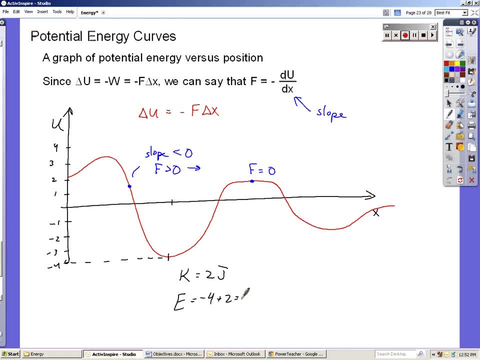 and so the total energy is negative. four plus two is negative two joules. That means if we look at the total energy for this particle, it's right there And that means: But this particle can never get higher than this point, than this level. 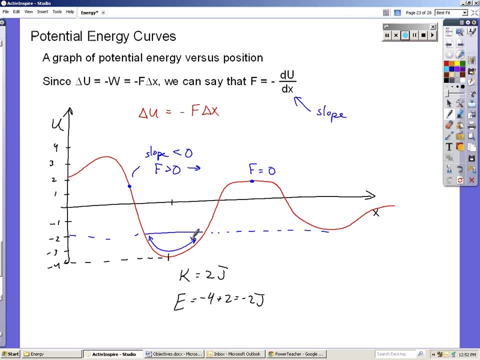 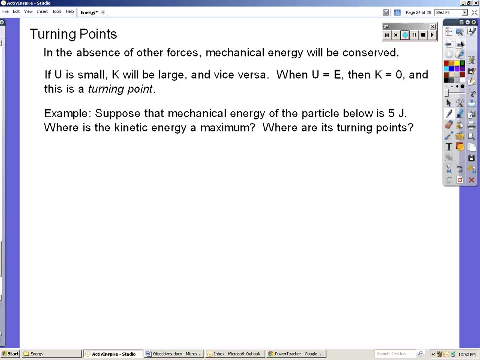 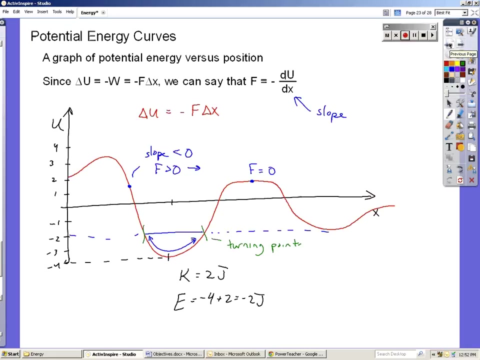 And so it's going to oscillate back and forth in that. well there, And we call these points here turning points, which is the subject of the next slide. Oh, there we go. Well, we kind of already did that. We should know what a turning point is, given a value of kinetic energy at a particular 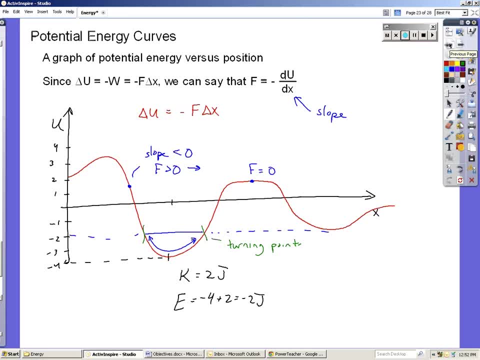 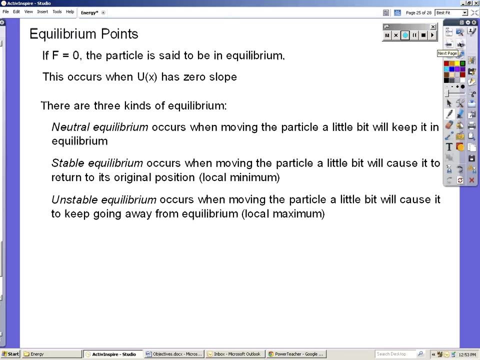 point, be able to calculate the total energy. that's what this number is. And then the turning points are places where the potential energy is equal to the total energy. In other words, kinetic energy is equal to zero. Now there's another concept called equilibrium points. 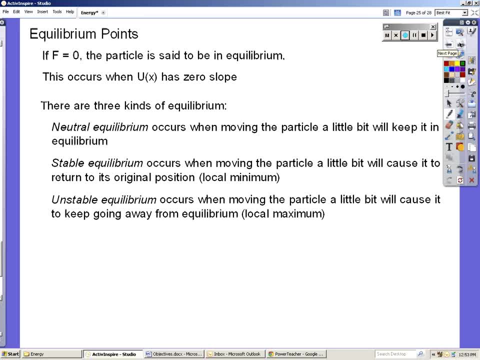 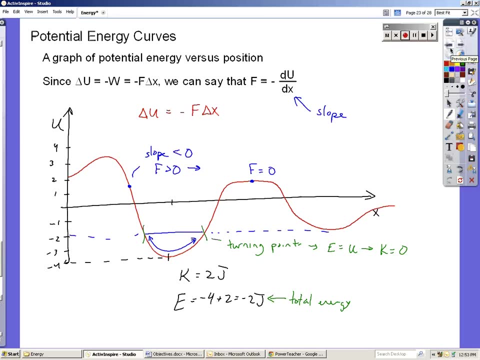 And remember equilibrium was a term we had for that indicated net force was zero, And so that's we're going to continue using that And that means the potential energy has zero slope at these points. And so we go back and we identify equilibrium points with orange. 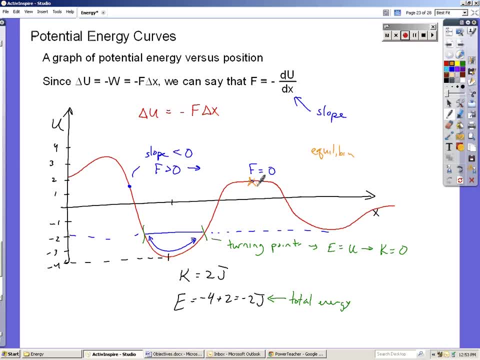 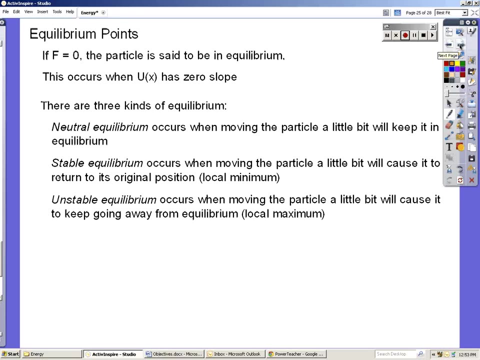 Here's an equilibrium point. Here's another equilibrium point, Another one And one more here. Notice that those are all minima or maxima on the graph. And there's a couple different kinds of equilibrium. The first kind is neutral equilibrium. 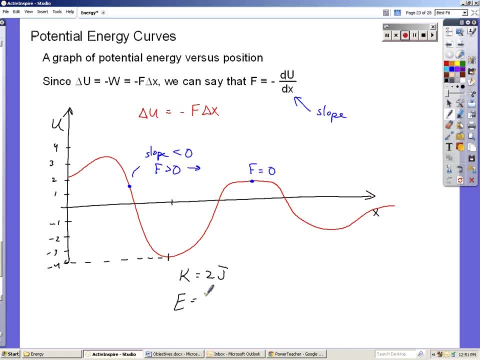 And so the total energy is negative. four plus two is negative two joules, And that means, if we look at the total energy for this particle, it's right there, And that means the potential energy of the particle is means that this particle can never get higher than this point, than this level, And so it's. 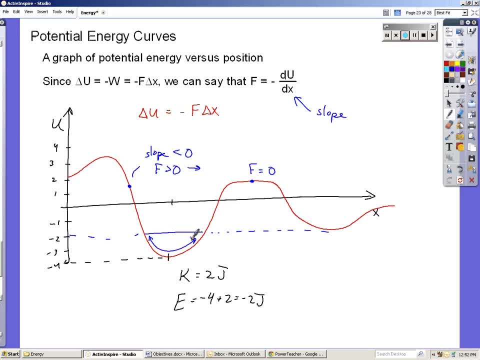 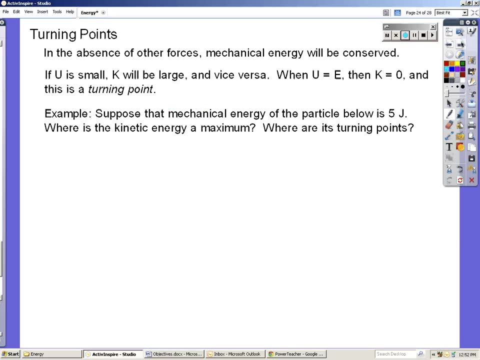 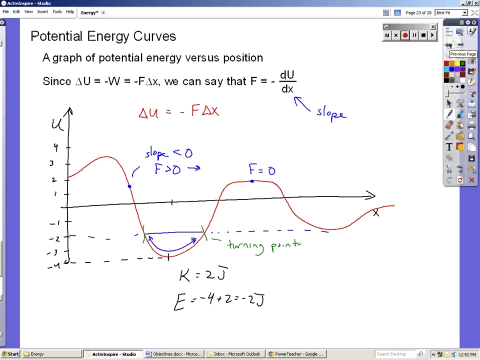 going to oscillate back and forth in that. well there, And we call these points here turning points, which is the subject of the next slide. Oh, there we go. Well, we kind of already did that. You should know what a turning point is. Given a value of kinetic. 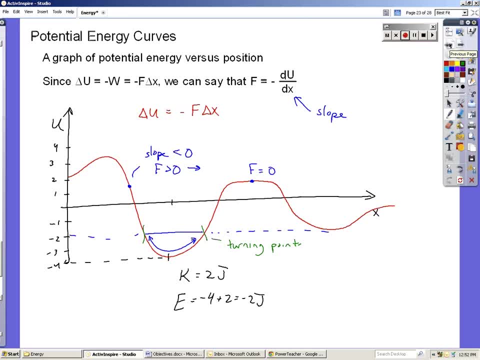 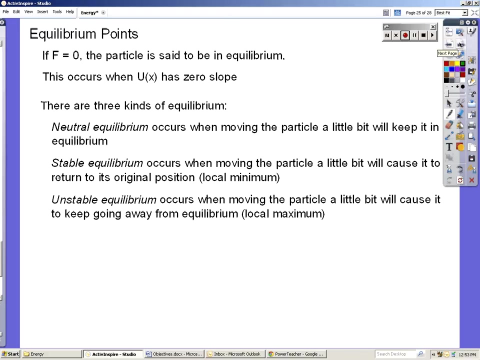 energy at a particular point, be able to calculate the total energy. That's what this number is. And then the turning points are places where the potential energy is equal to the total energy. In other words, kinetic energy is equal to zero. Now there's another concept called equilibrium points, And remember equilibrium was a term. 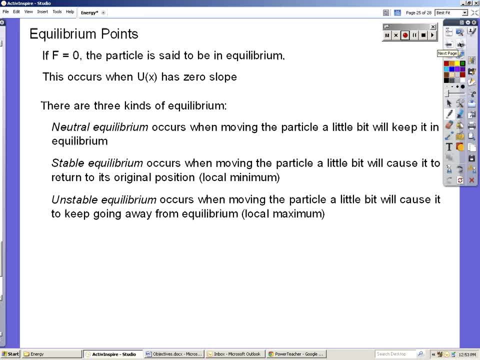 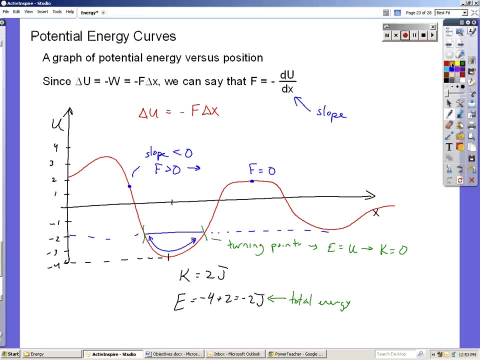 we had, for that indicated net force was zero, And so that's we're going to continue using that And that means the potential energy has zero slope at these points. And so we go back and we identify equilibrium points with orange. Here's an equilibrium point, Here's another equilibrium point, Another one And one more. 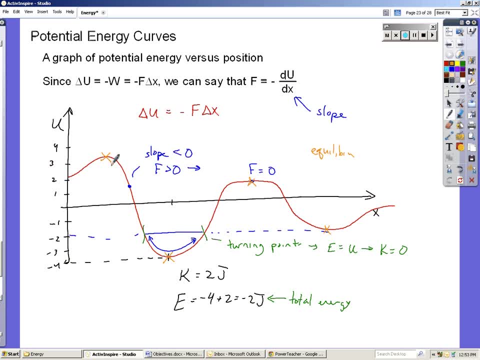 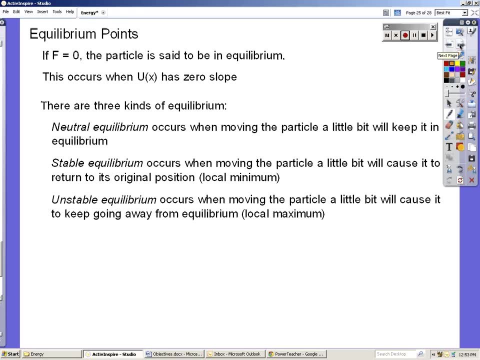 here- Notice that those are all minima or maxima on the graph- And there's a couple different kinds of equilibrium. The first kind is neutral equilibrium And that occurs when, if you displace the particle from equilibrium a little bit, it will still be in equilibrium. 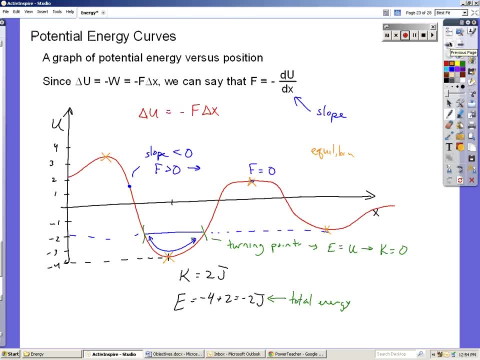 Basically that's where it's flat for a large distance. This is a neutral equilibrium point. The other kind of equilibrium are stable and unstable. Stable equilibrium means that moving the particle a little bit to one way, a little bit to the side, will make it come back And